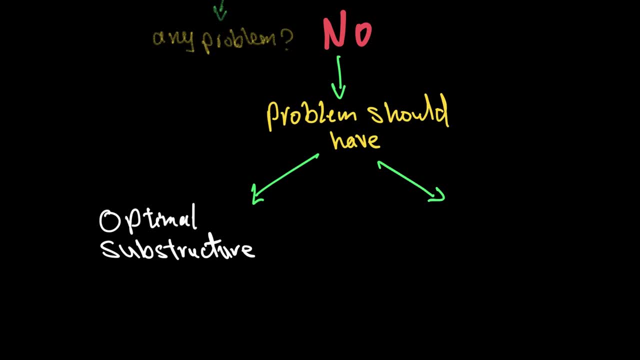 It should have optimal, superior and optimal solutions. These problems should be very accurate and efficient. So what you need to look for is the right answer. So when developing a program, try to find a model and also overlapping subproblems. Optimal substructure means the optimal. 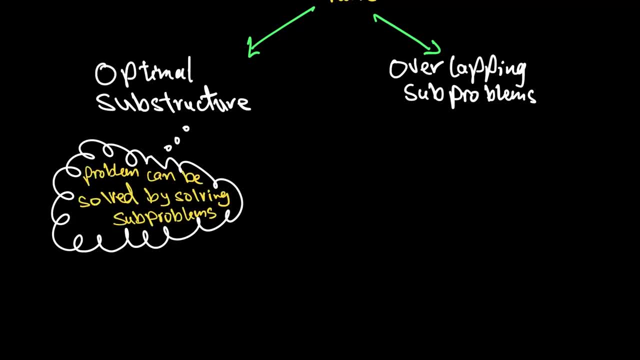 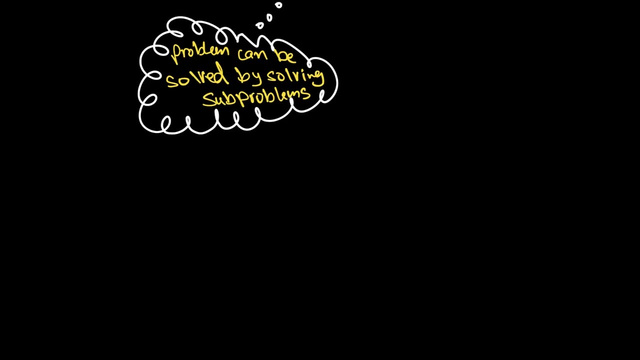 solution to the problem is the combination of optimal solutions to subproblems of that problem. This means if the problem can be divided into smaller problems and you managed to find the optimal solution to each of these problems, you will find the solution to the bigger problem. For example, if you 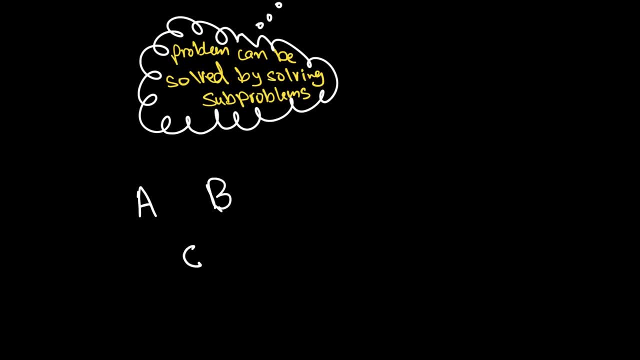 have got a few series- a, b, c and d- and you are trying to find the shortest path between a and D. If I tell you that the solution is a B, D, this means that there is no shorter path than a B D to reach from a to D. This means that the shortest 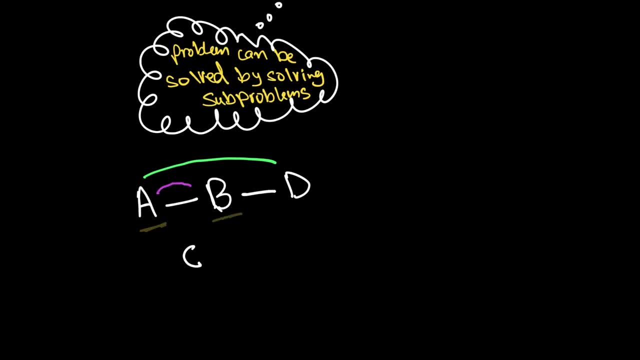 path between a and B is a- b, because if there was a shorter path from a to to B than AB, we would have taken it already in the solution. So here, in calculating the shortest path between A and D, we calculated the shortest path between 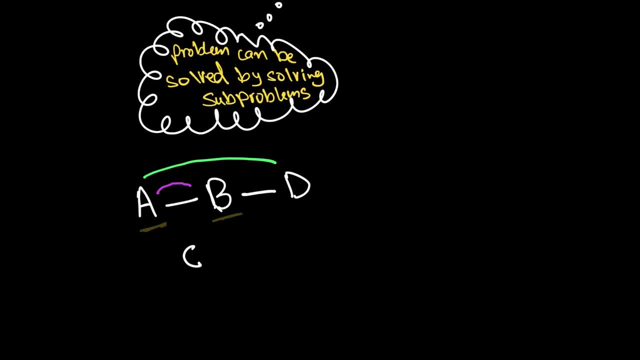 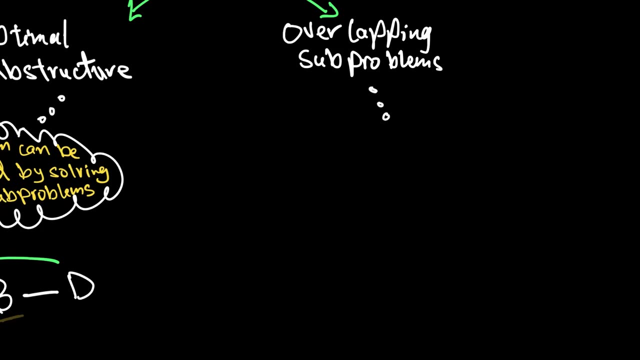 every city in between as well, and that is the optimal substructure. Dynamic programming can be used to calculate shortest path problems, although we will go through shortest path problems in another video. The second condition here is overlapping subproblems, which means that if you go through and you 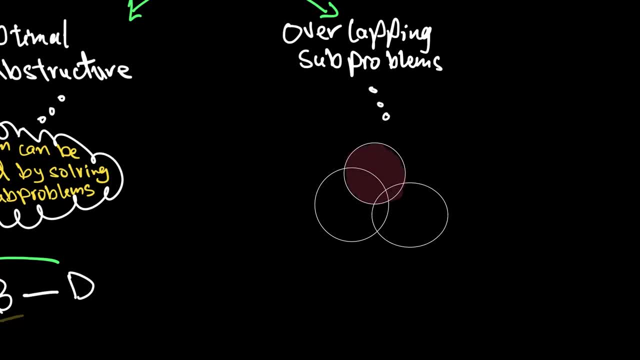 start to solve these subproblems, you will find yourself solving some of these subproblems over and over again. That was not clear to me. How am I gonna solve the same problems over and over again? This will make more sense when we give a real example. 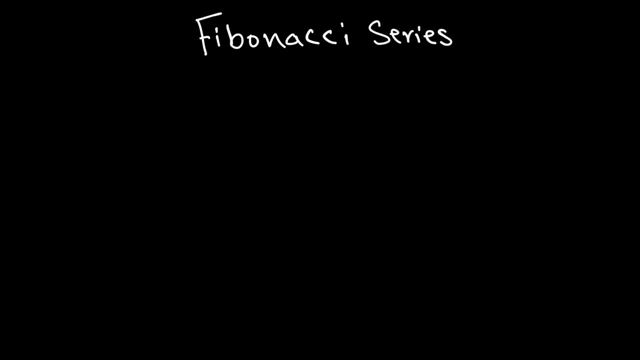 Let's use the Fibonacci series as an example. We have explained the recursive solution of the Fibonacci series in a video before. If you would like to check it out, you will find a link to it in the info box. A Fibonacci series is a series of numbers that look like this: 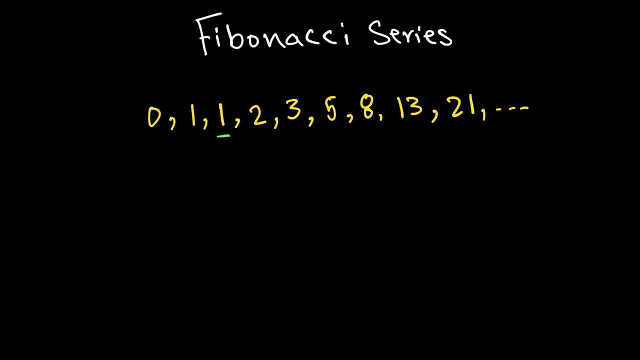 The first two numbers in the series are 0 and 1.. Then, starting from the third number in the series, each number is calculated as the sum of the previous two numbers. So 1 is the sum of 0 plus 1,, 2 is the sum of 1 plus 1,, 3 is the sum of 2 plus 1, and so on. 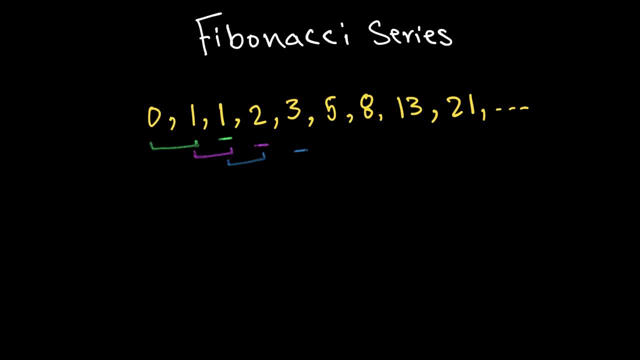 Fibonacci series is a perfect candidate of a dynamic programming solution. But why? First, because it satisfies the optimal substructure condition. To calculate each number in the series, you will sum up the previous numbers together, And to calculate those, you will sum up the previous numbers together, and so on. 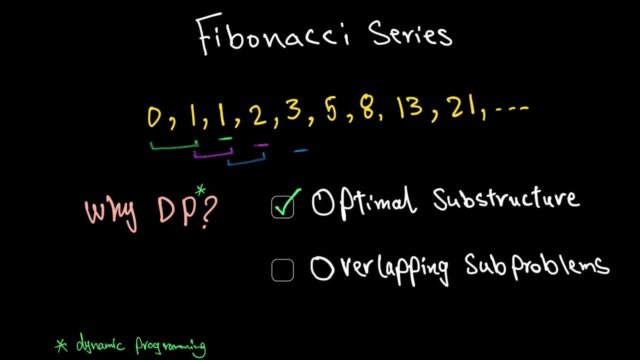 So the solution of the problem depends on the solution of subproblems. Second, did you notice the overlapping here? For example, We have two numbers in the series starting from 0. So to get the solution of the series at index 5, we need to calculate the number at index. 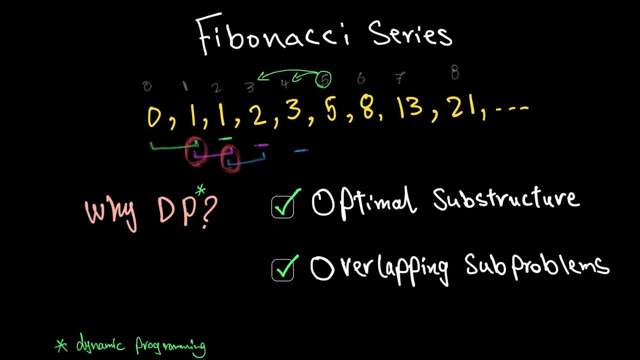 4 and the number at index 3 and sum them up together. But to calculate the number at index 4, we need to calculate the number at index 3 and the one at index 2 and sum them together. Do you see the overlapping? 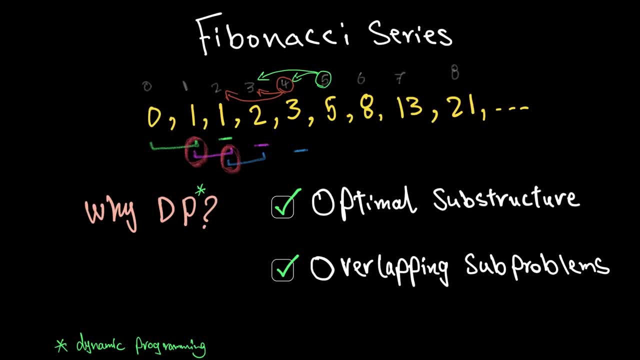 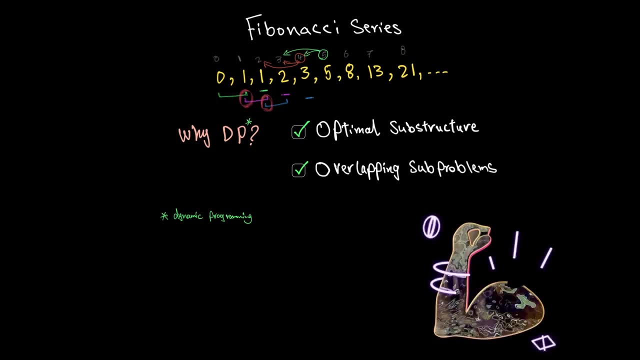 This overlapping can be hard to recognize at first, But if you try to spot, the more you get exposed to dynamic programming problems. You will be able to sense the pattern in the problem and say, aha, this is a dynamic programming problem. 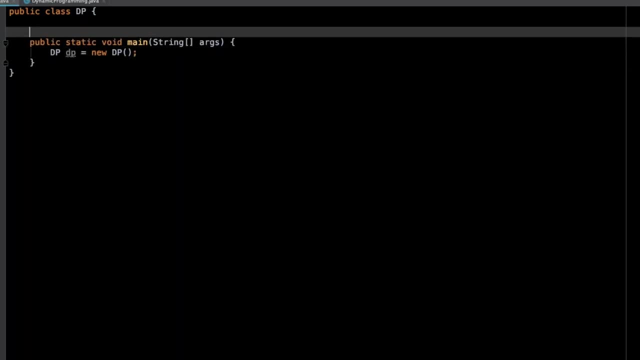 Let's code the solution of this problem. The most natural solution that comes to mind is the recursive solution. Again, we explain that in detail in a video in the info box, so check it out if you want more details about the recursive solution. 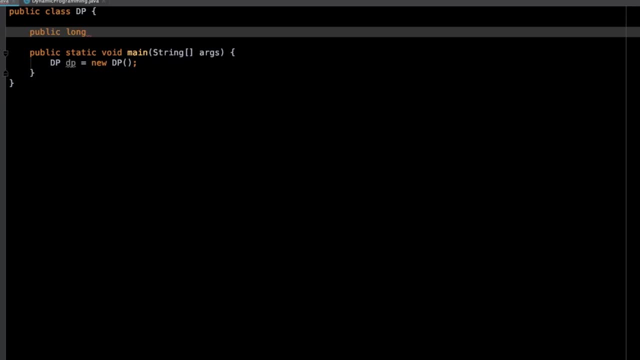 Let's create a function that takes care of the recursive solution. Let's create a function that takes care of the recursive solution. Let's create a function that takes care of the recursive solution. We need to map it using a similar algorithm with index n as a parameter. 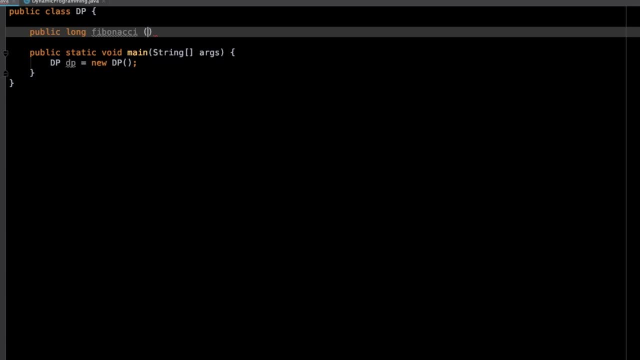 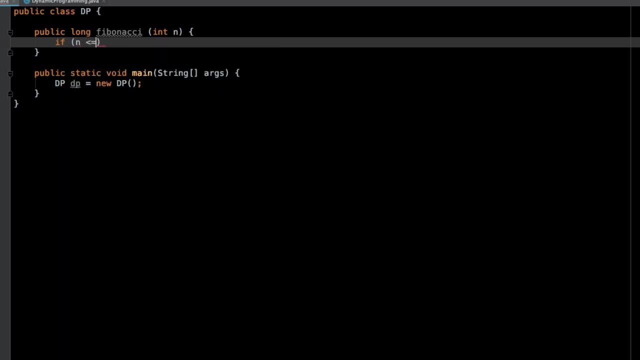 The index n is an integer that represents the index for which we want to calculate the Fibonacci series. We know that the Fibonacci of 0 is 0, so let's reflect that via an condition. Fibonacci of 1 is also 1.. Let's add an condition for that. 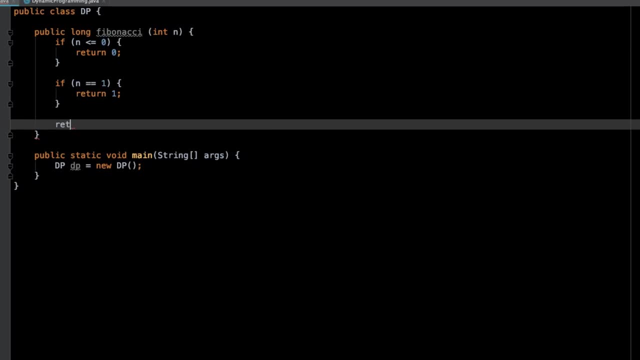 Otherwise, the solution should be the Fibonacci of the previous two numbers summed up together. If we know the Fibonacci of 0, then it is equal to the Fibonacci of f. So let's stick that distribution to our definition of f. So let's stick that distribution to our definition of f. 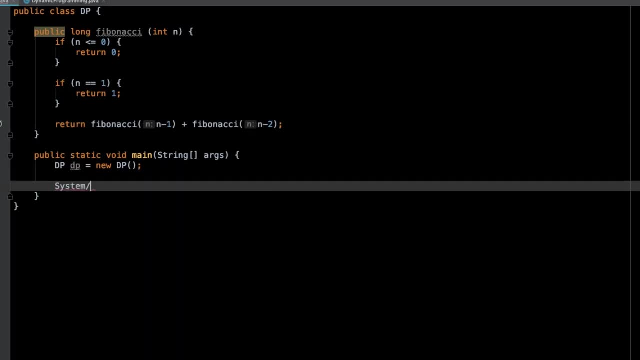 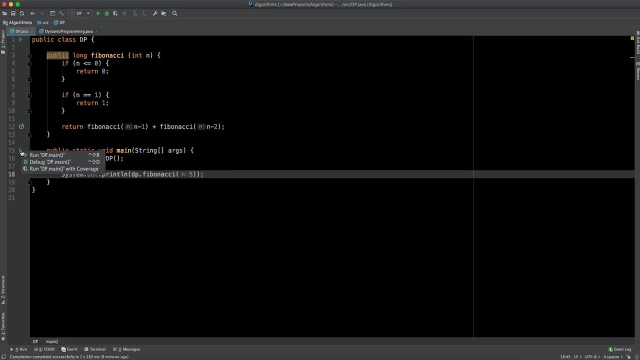 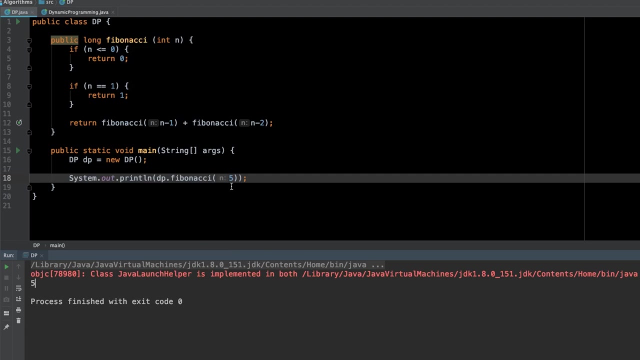 Let's try that. Let's get the Fibonacci of 5.. Let's add that. Let's add that. That's 5, correct. Now let's get the Fibonacci of 7.. That's 13,, also correct. Now let's get the Fibonacci of 50.. 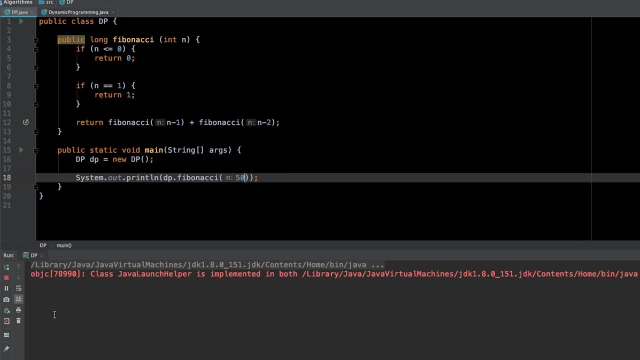 Oh, it is taking so much time to calculate Fanto. can you guess why? Of course I can. that's because of the overlapping problem you mentioned. I think we are calculating certain Fibonacci's multiple times right, Absolutely right. Let's trace the solution on paper. 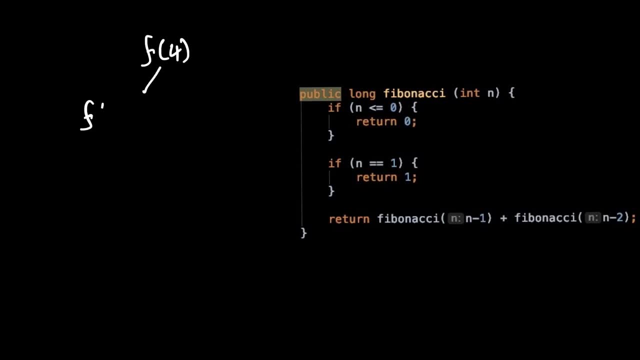 Let's say we need to calculate Fibonacci of 4.. Fibonacci of 4 is Fibonacci 3 plus Fibonacci 2.. Fibonacci 3 is Fibonacci of 2 plus Fibonacci 1.. Fibonacci of 2 is Fibonacci of 1 plus Fibonacci 0.. 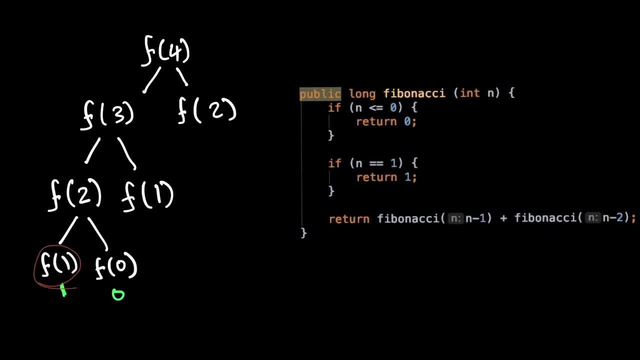 Fibonacci of 1 is 1,, Fibonacci of 0 is 0. Here is the overlapping problem that we have. But what if we save the solution of Fibonacci 2 somewhere and use it when we need it? Oh Fanto. 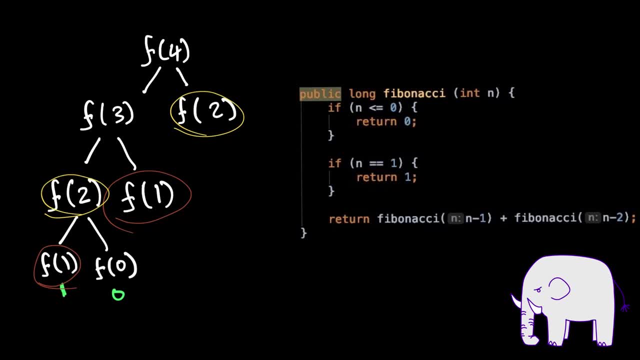 I don't know why you are here. You already know everything. That's very correct. We can save the solutions to Fibonacci's that we already calculated in an array and check in that array if we have the Fibonacci number before we calculate it. 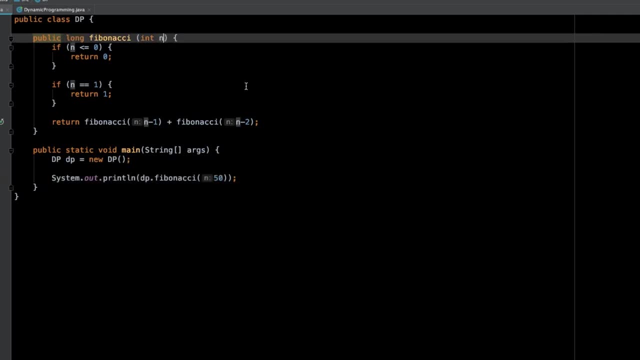 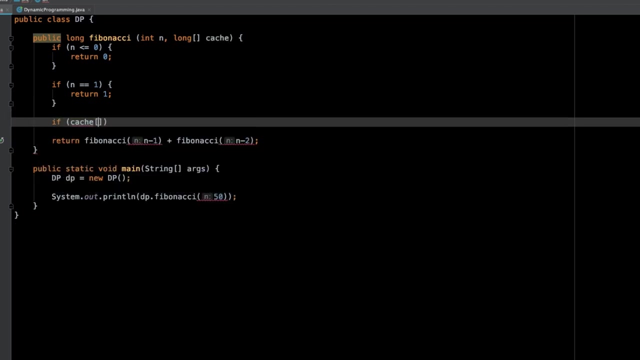 Let's try that. I will add here an array called cache. This array will have n plus 1 integers. We will pass that array to the function, Then check if cache of n exists. This means that we already calculated the number before. 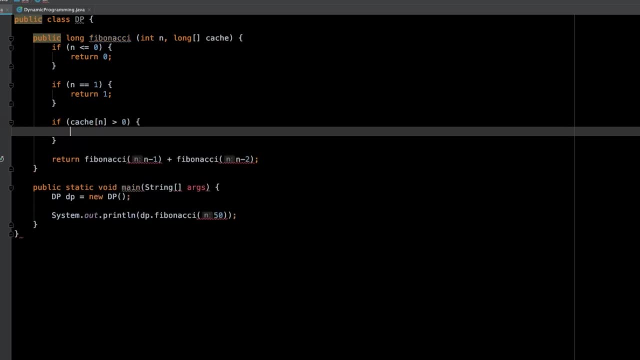 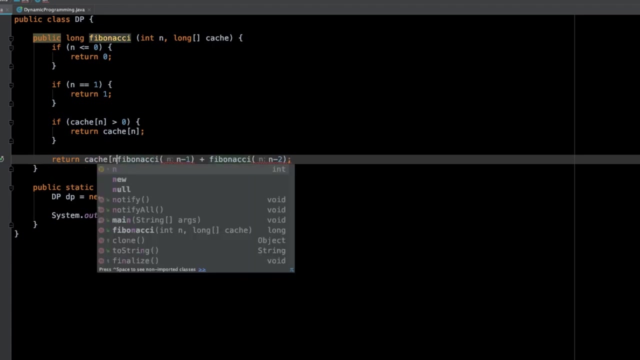 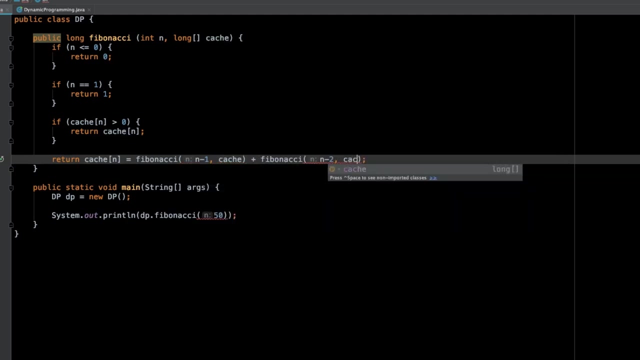 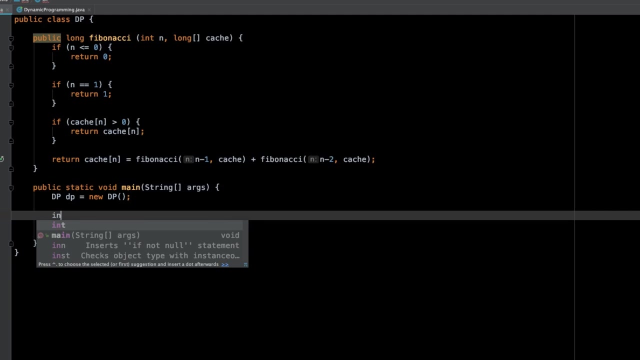 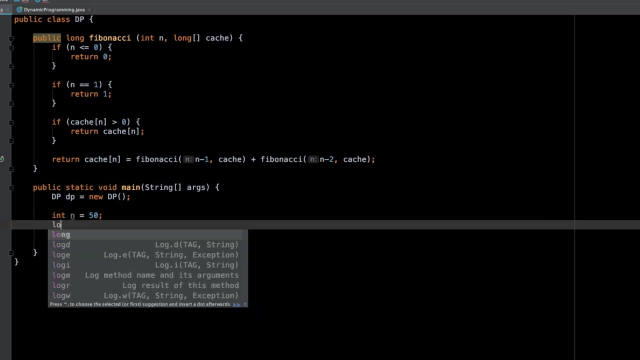 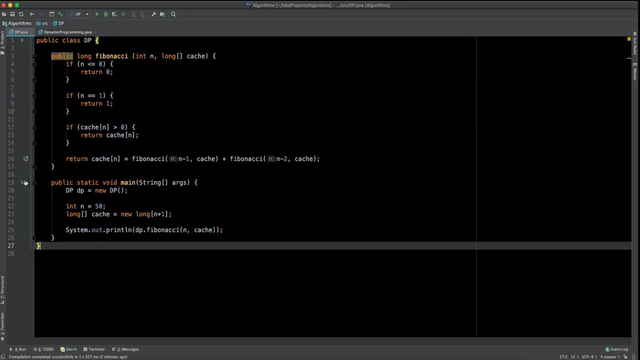 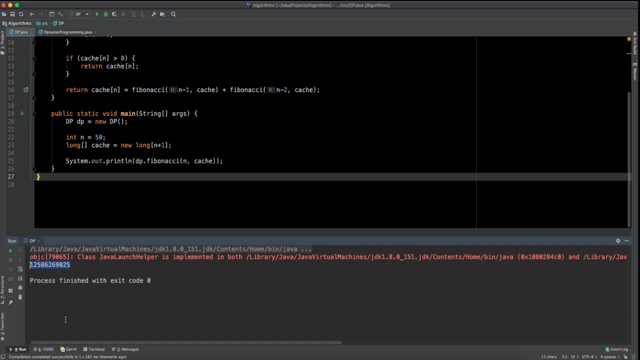 Then we return it right away Here. we need to store the result of n in the cache array, And that's it. Now let's try to get the Fibonacci of 50.. Oh, that's so fast. Obviously, the caching approach improved the performance significantly. 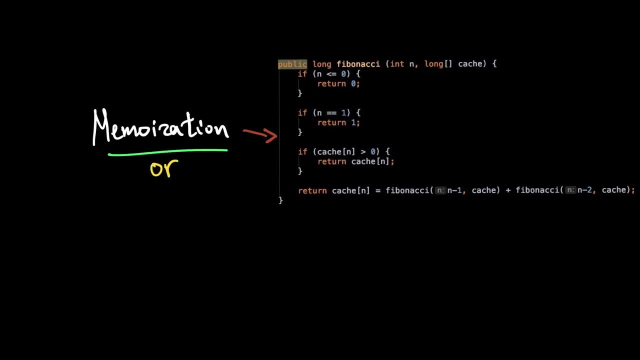 This approach that we use now is called memoization or top-down approach. Okay, we are saving the results in order not to recalculate them, So memoization makes sense, but where is the top-down in that? It is top-down because we started from the end result. 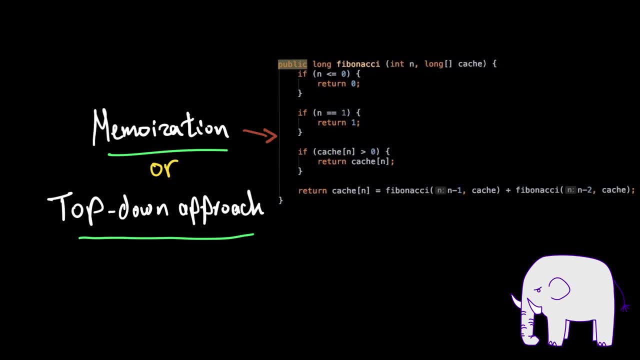 The bigger problem And then divided that into smaller problems. I'm still not convinced. Okay, let me first introduce you to the other approach and this will make it more understandable. Sometimes you just understand the concept by understanding the opposite of it, you know. 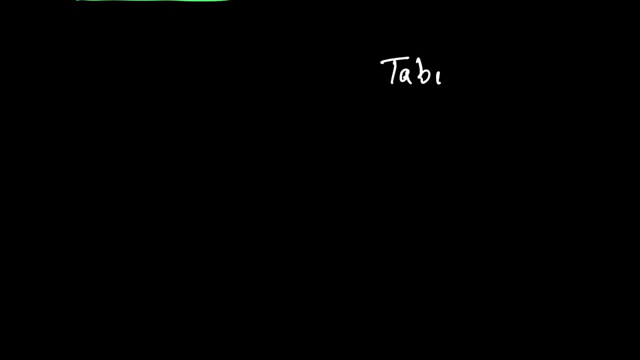 Alright. The other dynamic programming approach is called tabulation or bottom-up approach. With that approach you start from the bottom And gradually build your way towards the bottom. Let's have a look again at the Fibonacci series. If we know that the first two numbers in the series are 0 and 1, now to get the Fibonacci. 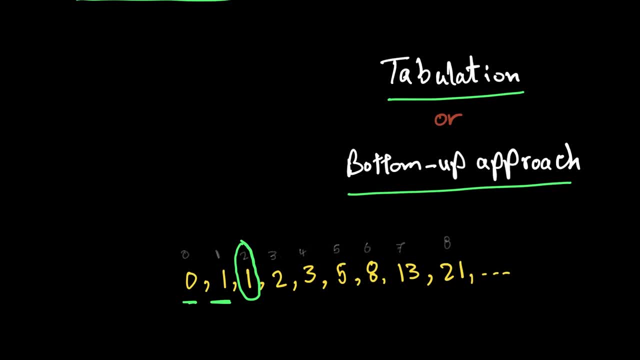 of 2,, which is the third number here. it is the sum of the previous two numbers. If we start a loop from here on and store the calculations in an array, as we did it with the memoization, this will be the tabulation solution. 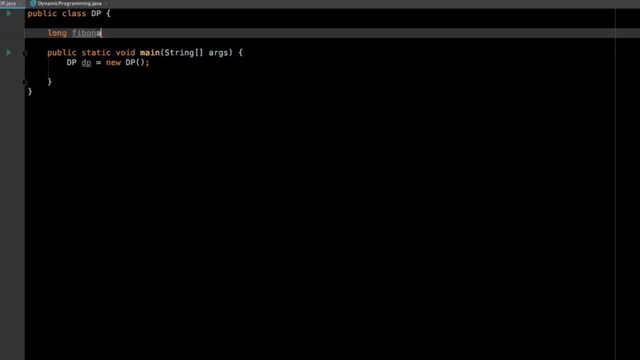 Let's try that down. We create our fib function First. we create an array which has a length of n plus 1.. We know that the Fibonacci of 0 is 0 and the Fibonacci of 1 is 1. So we set them in the array. 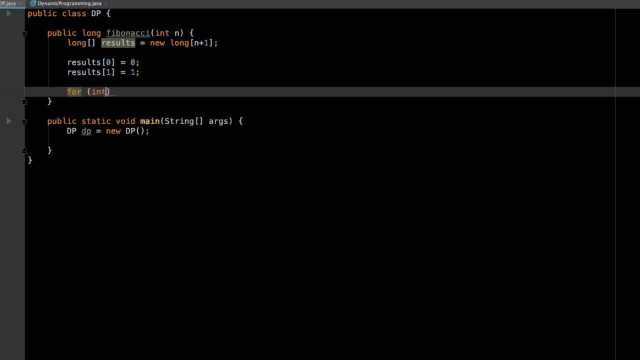 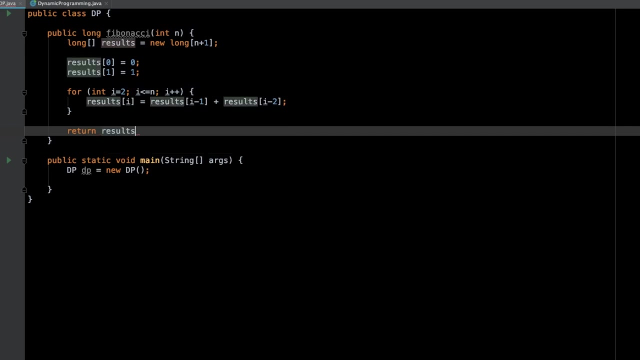 Then we loop, starting from 2, and start calculating the missing Fibonacci up until the number that we are interested in, which is n, And then we return the Fibonacci of n from the array. That's tabulation. Now, let's try that. Let's get the Fibonacci of 5.. 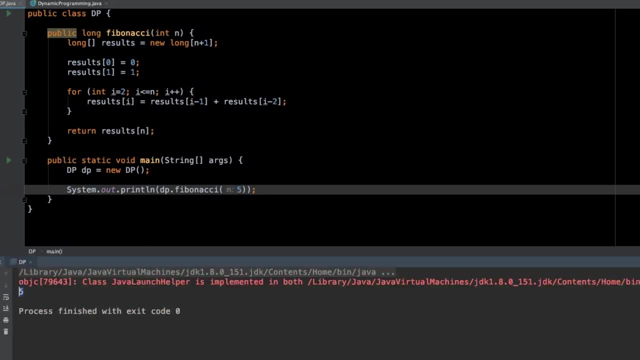 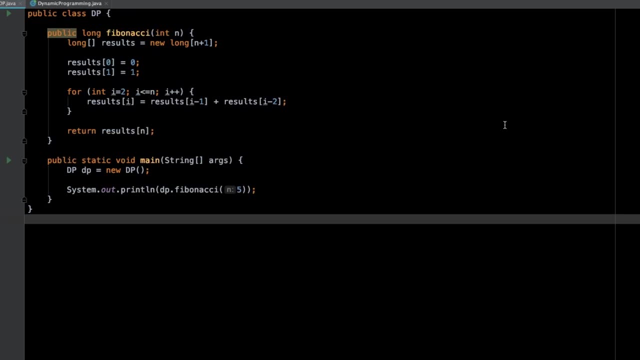 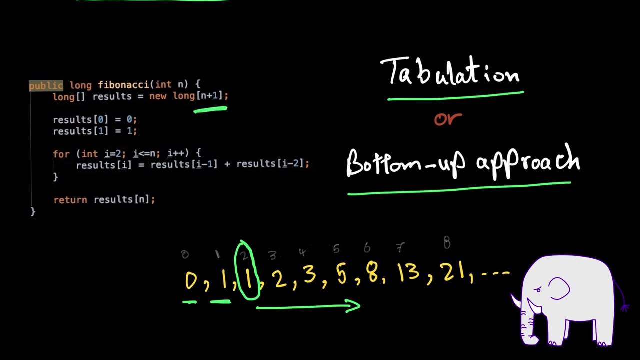 That's 5.. Correct, Depending on your preference. you might find tabulation even simpler than using recursion, And I tend to find it simpler, actually. Okay, everything is fine, but why we created an array with size of n plus 1?? 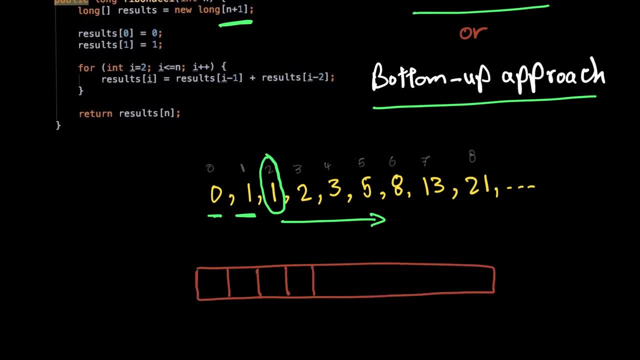 Because array indices start at 0, and we want to store the result up until the number n. If you have an array of length of n, the index of the last element in that array will be n minus 1.. But since we want to store the result of n, we need one more element to the array. 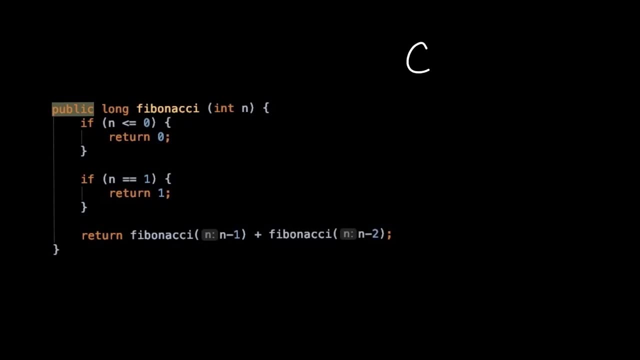 Now let's calculate the time and space complexity. Let's start by the recursive variation first. As always, please pause the video and try to calculate the time and space complexity yourself first. Alright, actually it is easy to calculate the complexity in here. 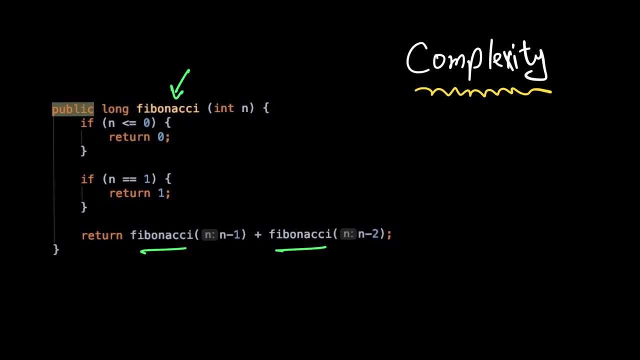 In each call to the Fibonacci function, Let's add a new function. call the Fibonacci function two times, And in each of these calls we call the Fibonacci function two times, and so on. This means two times, two times two, and so on. How many times are we going? 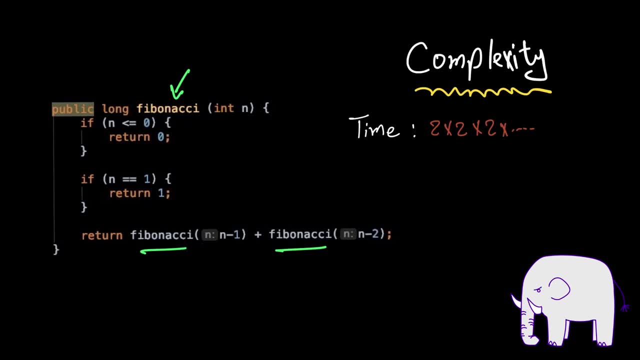 to do that. I think we will do that n times because once we reach zero or one, we will just return the solution which we already know: either zero or one. So complexity is O of two to the power n Just make it a rule. Time complexity of a recursive function is the number of times you